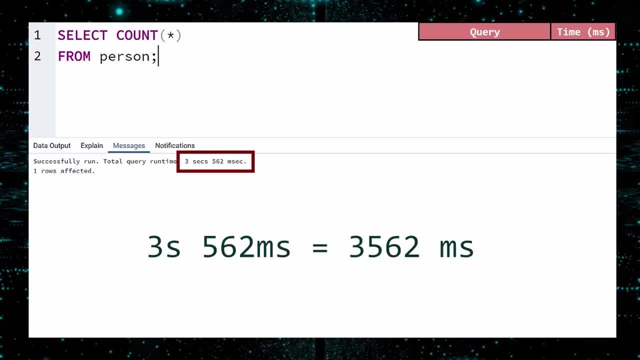 Or 3,562 milliseconds. Let us put this query and the time required in our table. As another speed test count: the number of people with the last name Smith Execute Over 100,000 Smiths And the query took 4,261 milliseconds. 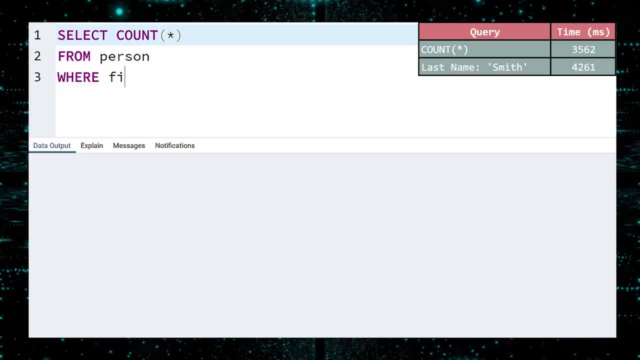 For a second test, count how many people are named Emma Execute, Nearly 50,000.. And note the time: 4,066 milliseconds. What if we count the number of people born in May 1980?? For this we will use the BETWEEN operator. 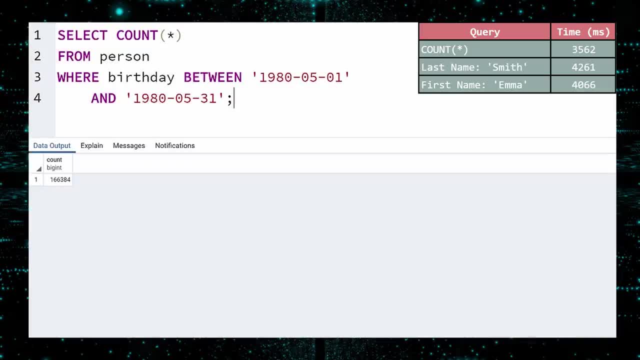 Execute 166,000.. And the query took 4,480 milliseconds. A pattern is starting to emerge. Let's quickly gather a few more speed samples. How many Michaels are in our database? 4,127 milliseconds. How many people have the last name, Hawkins or Snow? 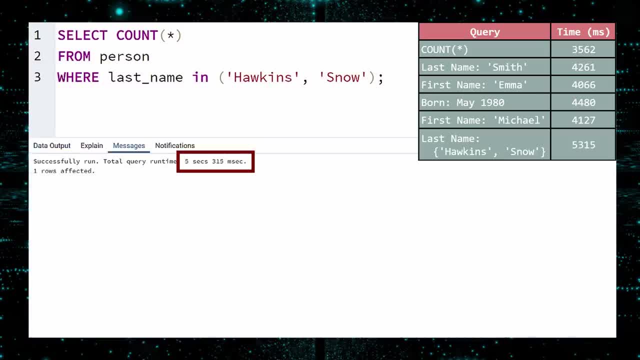 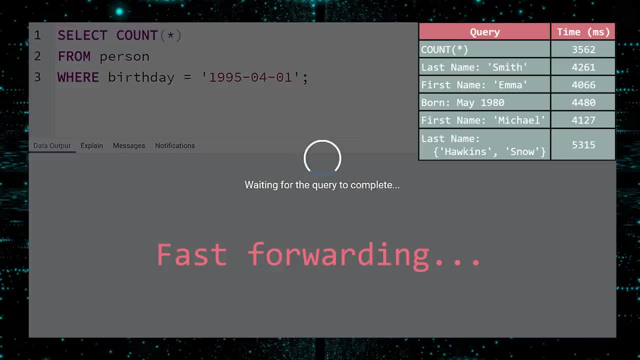 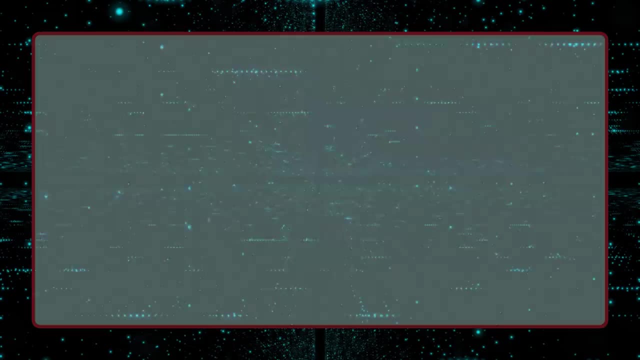 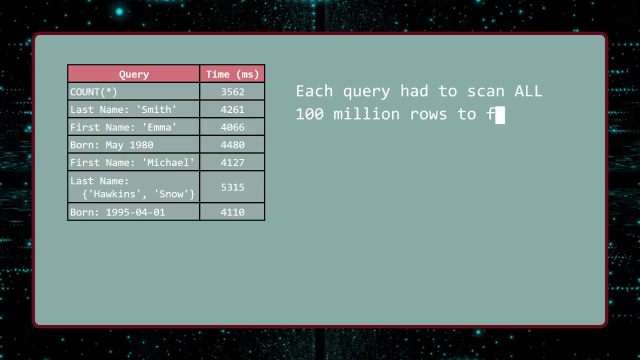 5,315 milliseconds. And how many people were born on April 1, 1995? 4,110 milliseconds. We ran seven queries and the execution times were all very similar. This is because, in order to answer each query, the database had to scan all 100 million rows. 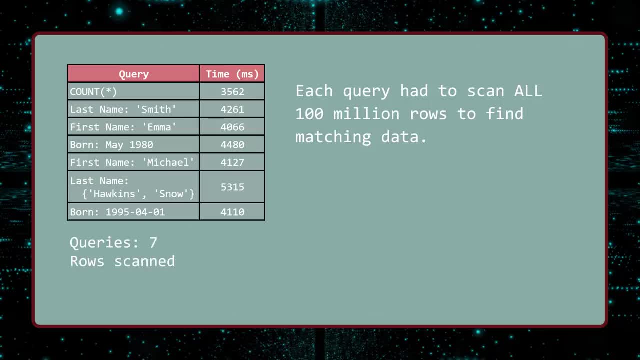 to check each record for a match. Our seven scans of the entire table took a combined total of 29,921 milliseconds. This means on average, my workstation was able to scan 23,394,940 rows per second. While this may seem fast, we can do better. 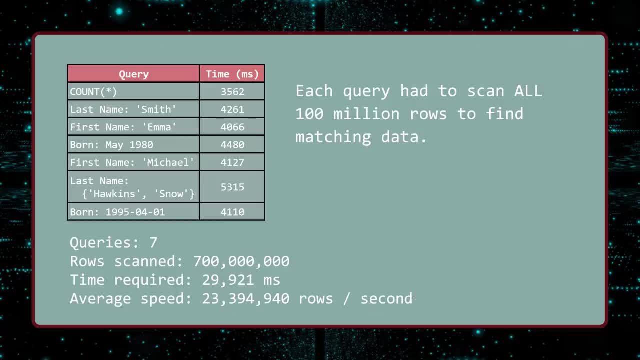 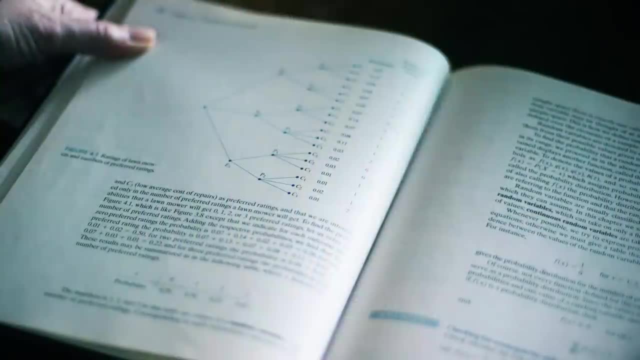 Much better, And we will do this by building an index. The name index was chosen because of how an index works in a book. For example, if you want to learn about normal distributions, you would not flip through your entire math book page by page. 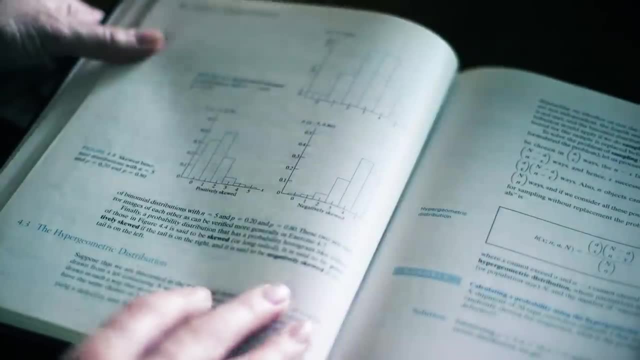 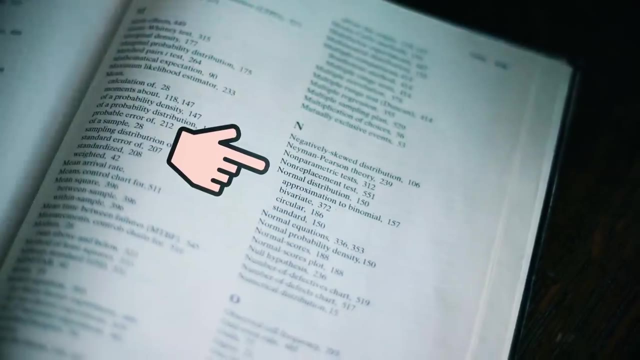 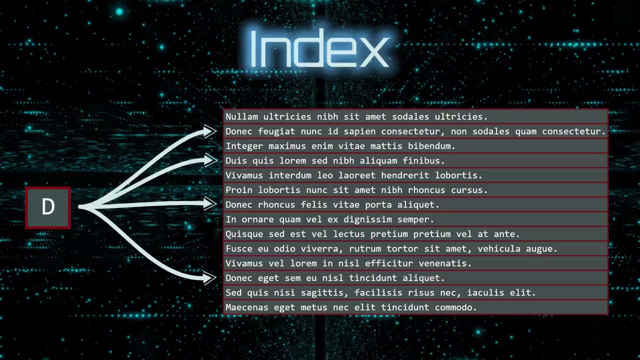 scanning for the term normal distribution. Instead, you would go to the index, find the term normal distribution and you would see the list of pages. This technique is used by databases. When you create an index, the database will generate a method to rapidly find data based on one or more columns. 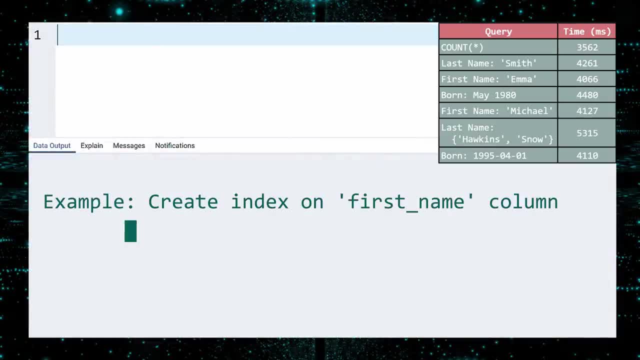 As our first example, let us create an index on the person. To do this, write, create index and then give your index a name. There are many different naming conventions that you can use. The important thing is to be consistent. We will use the table name, followed by the field name. 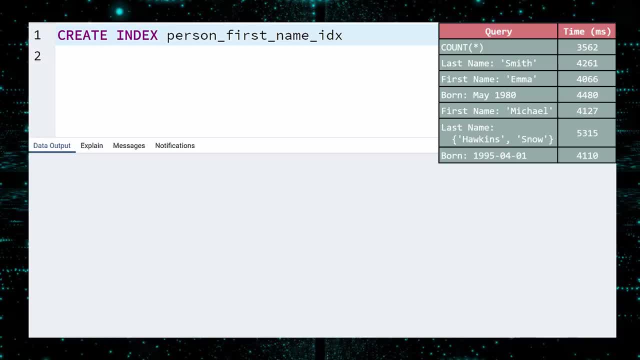 then add idx to indicate this is an index. Next write on, followed by the table name. Inside parentheses, write the columns to include in the index. We will start simply and create an index. for the index We will use the first name column. 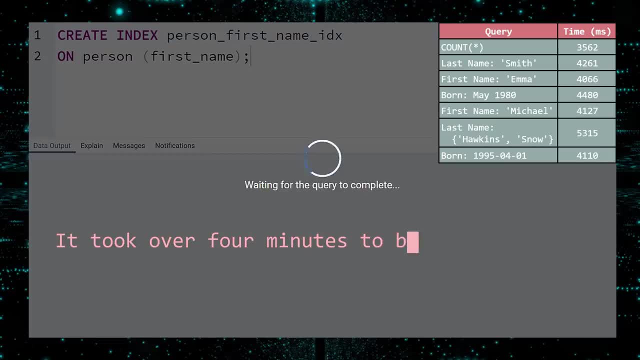 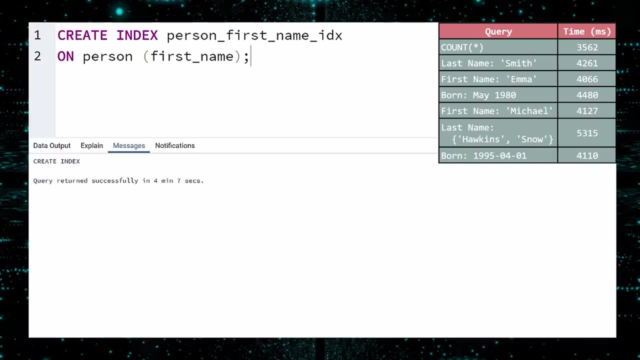 Execute. That certainly took a while. Remember the database had to scan 100 million rows and build a first name index from scratch. Let's test our new index by repeating an earlier query where we counted the number of people named Emma. Execute. 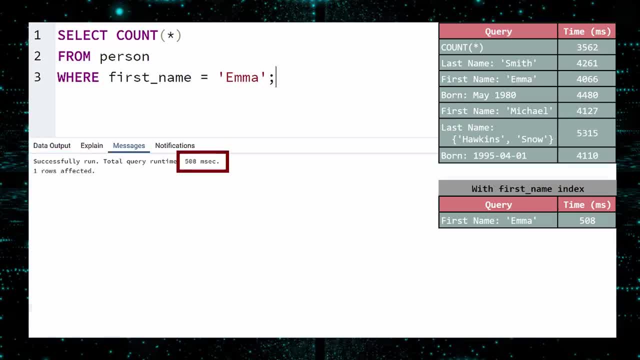 This time it took only 508 milliseconds. If we repeat the count of people with last name Smith, it takes 4,415 milliseconds. What's going on here? This is about as long as it took last time. It did not speed up because our index was built for the first name column. 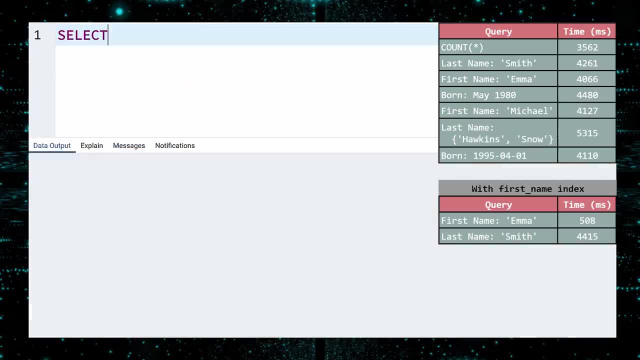 The last name was not indexed And, as you might suspect, if we search for people born on April 1, 1995, the query should not run any faster than last time. Execute 4,011 milliseconds, No real change. 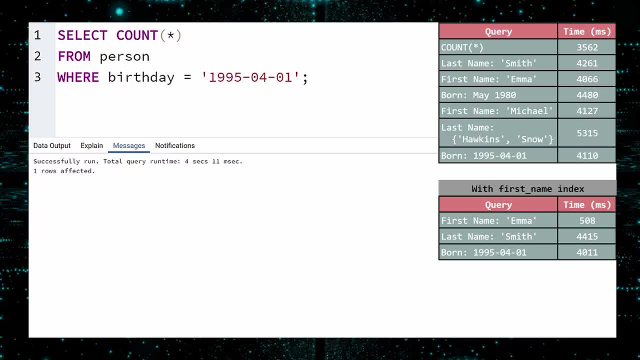 Our index improved the speed of searches by first name, but had no effect on queries by last name or birthday. However, there are other queries where the first name index will improve performance. For example, count the number of people named Julie Andrews. Execute. 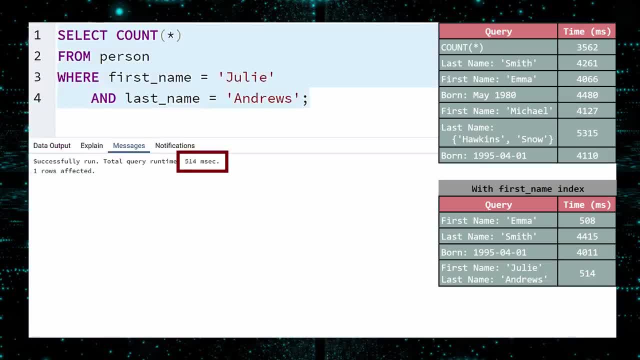 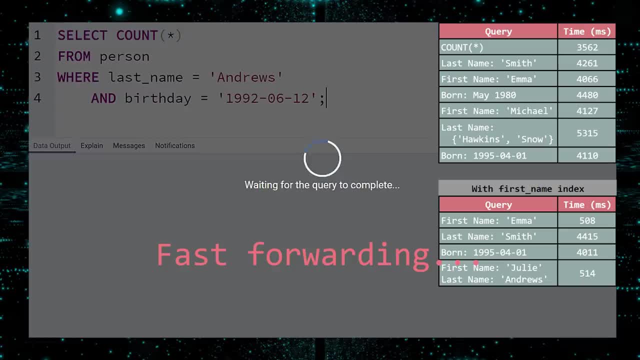 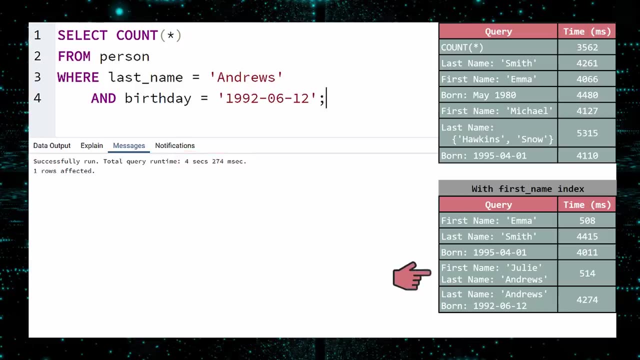 This ran in just 514 milliseconds. By contrast, if you count people with last name Andrews and born on June 12, 1992, it takes 4,274 milliseconds. The full name query benefited from the first name index because the database was able to use it to quickly find all the Julies. 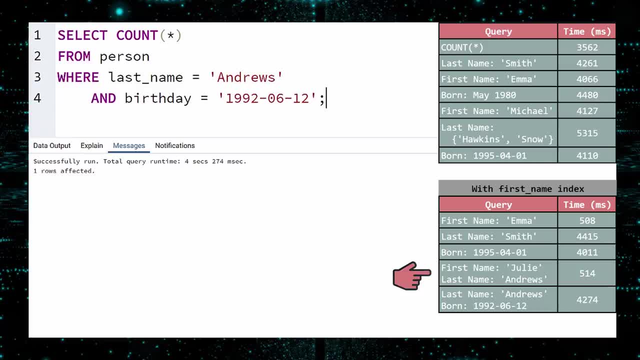 From this smaller set of records. it then completed the job by finding people with last name Andrews. The second query, however, had no index to help. It had to perform a full scan of the table to find all people with last name Andrews and then find those with a matching birthday. 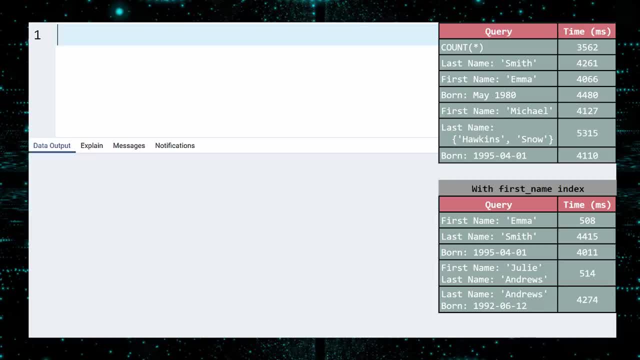 Fortunately, databases are clever about how to use indexes. For example, if you count the number of people born on October 31, 1985 with a first name of Mia, it executes quickly 512 milliseconds. But why Wouldn't the database first scan all rows? 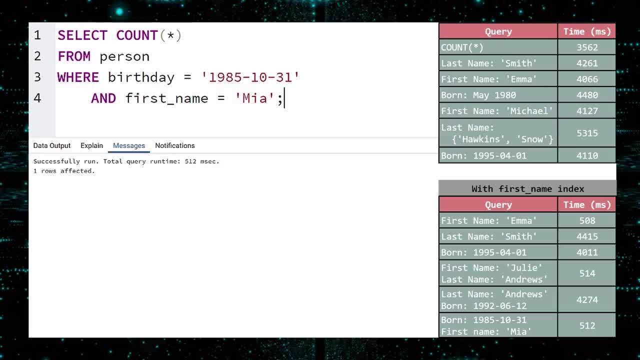 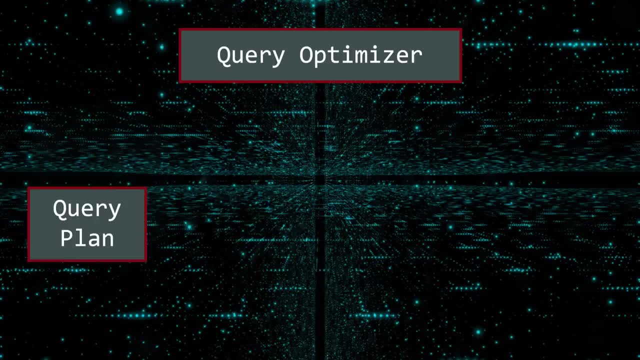 to find people with a matching birthday and then filter by first name. No, Just because we wrote it in this order does not mean the database will do its work in that order. The database considers all possible ways to execute your query, then chooses the optimal path. 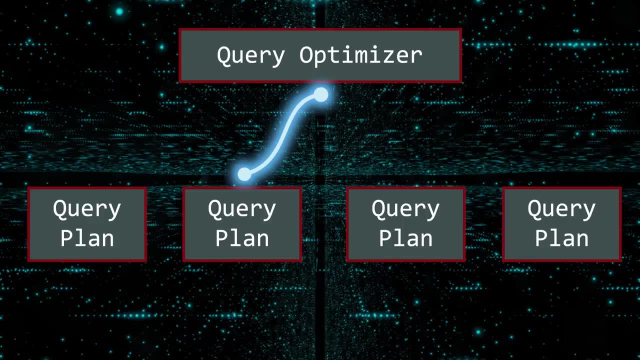 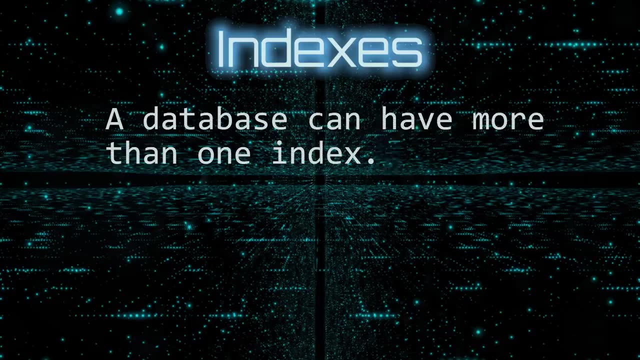 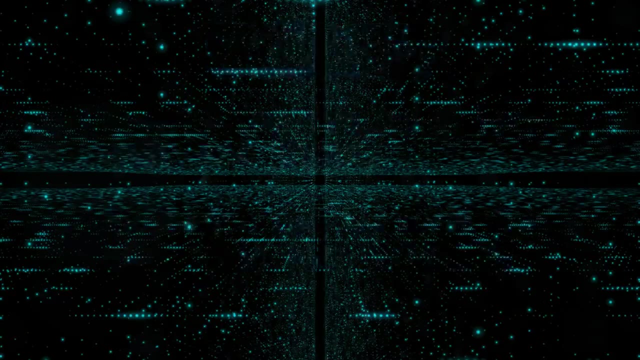 We call each possibility a query plan and the query optimizer picks what it thinks is best. You'll be happy to know. a database can have more than one index. Better still, each index can be created using more than one column. Let us create a multi-column index. 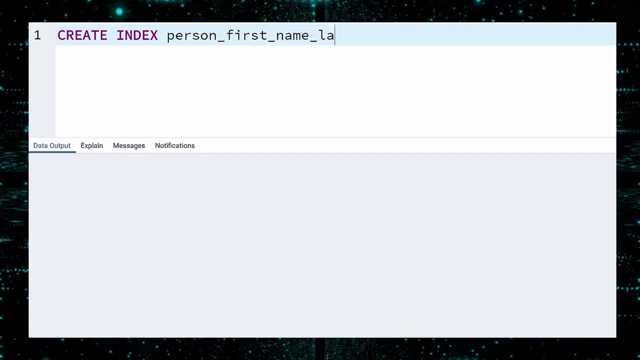 Write create index, then an overly long but descriptive name. Next write on, then the table name. In parentheses list the columns you want to go into this index. Important note: the order matters. Think of this as sorting the data first by last name. 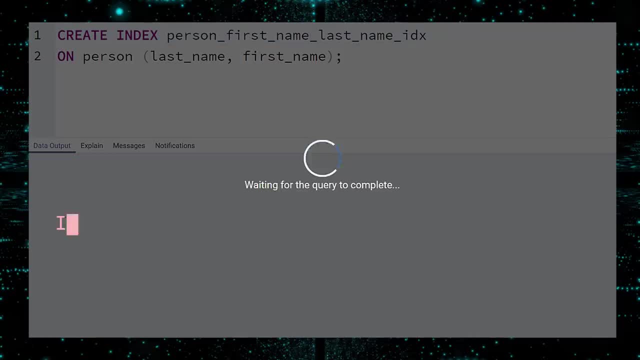 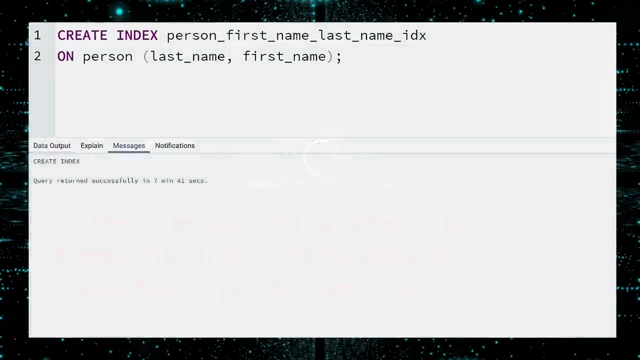 then by first name: Execute. It is now time to take this new index for a test run. How many people named John Williams are in the database? Execute? There are 36 people and it only took 27 milliseconds to run this query.